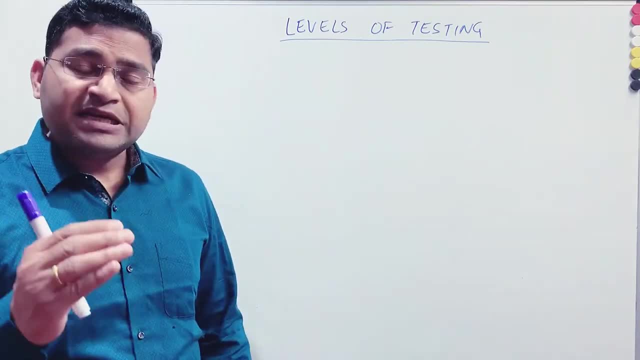 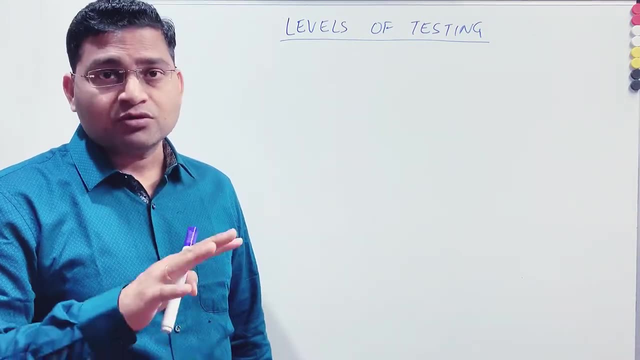 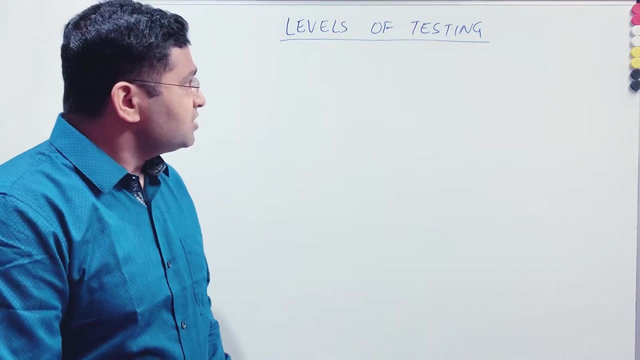 tutorials. So, when we talk about the levels of testing, there are mainly four levels of testing in software testing. okay, So that's the important thing to remember: four levels of testing And all the types of testing can be fit within those four levels, right? So the first level of testing is: 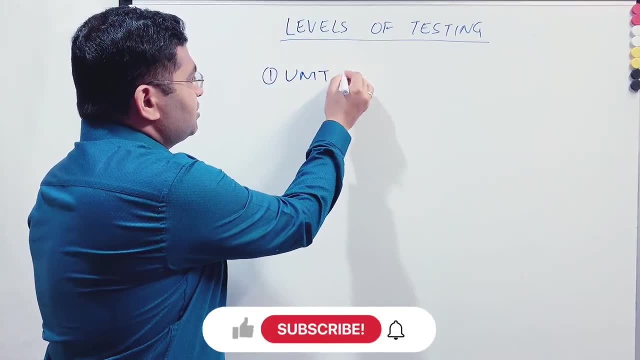 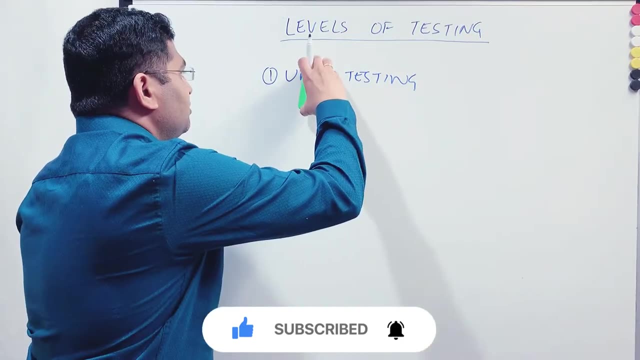 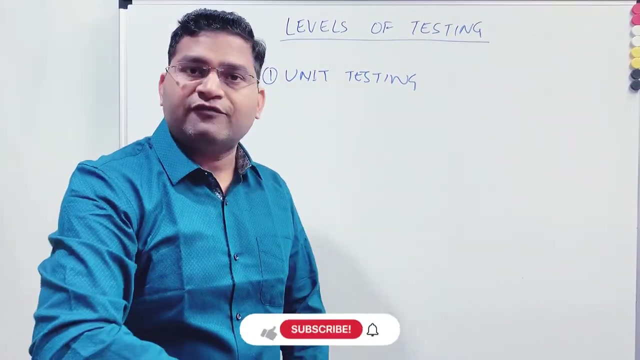 unit testing. all right, so unit testing. so what happens in unit testing? so say, for example, you are building the e-commerce application, right? so e-commerce application will have a lot of functionalities. so we'll take a login page example, which is the simplest to explain and understand. 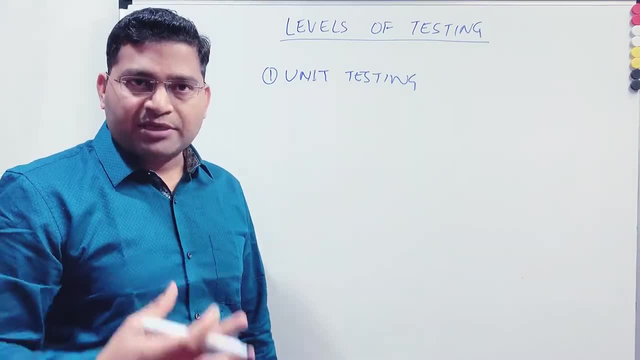 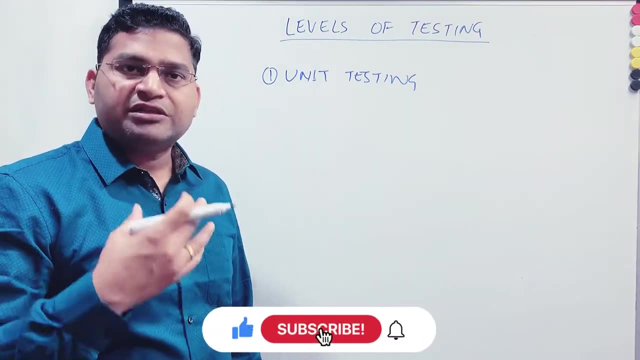 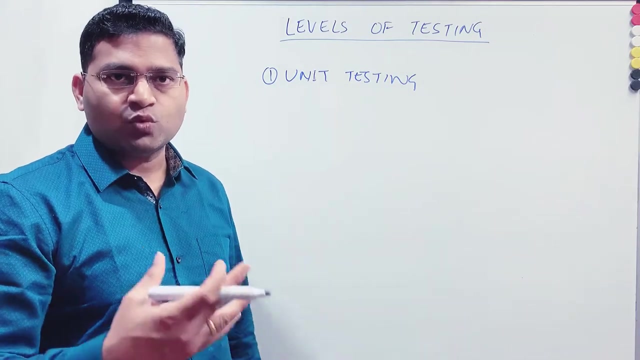 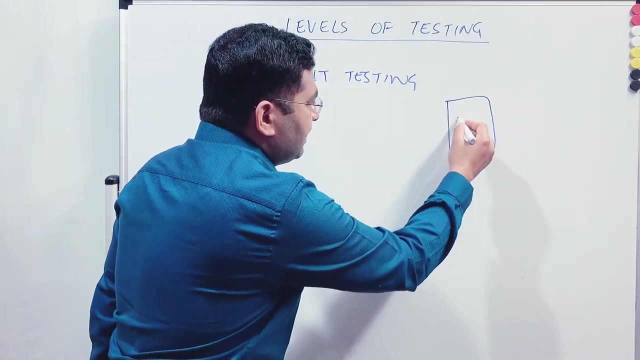 right. so login page will have the username and password fields and the login button. so in that particular case, when some developer starts developing that login page functionality or the login functionality, so if he is a ui developer, so what he will work on is he'll work on the first page and that page will have this login username and password and the login button. 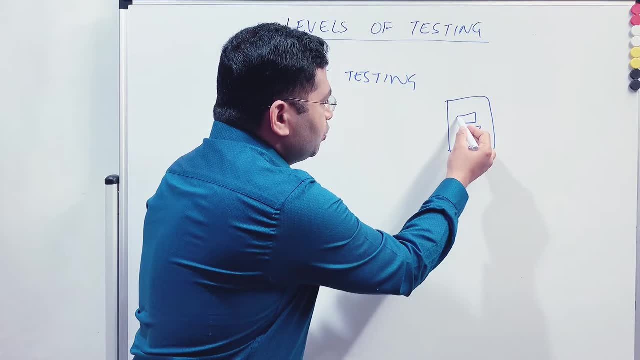 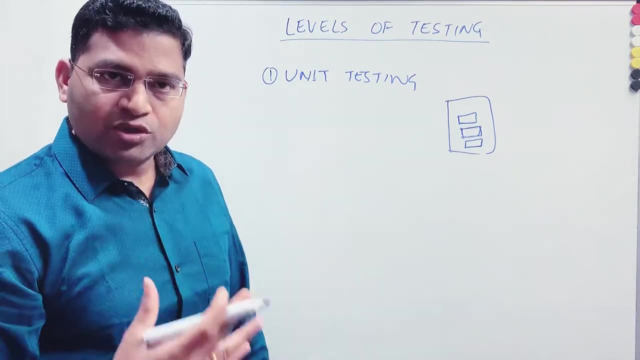 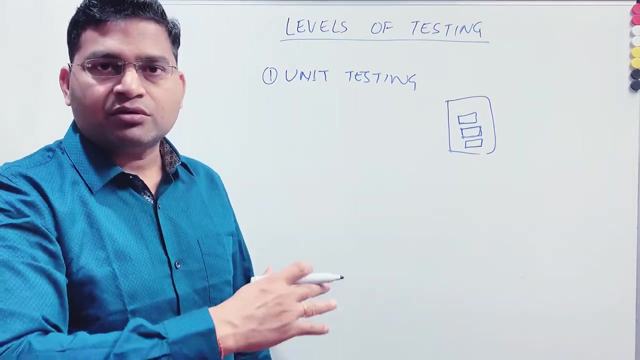 right. so when he works on this username and password field there will be some you know restrictions or limitation or requirements, basically in terms of username and password. say, username cannot be more than you know 50 character or 100 characters. password should should have you know a special 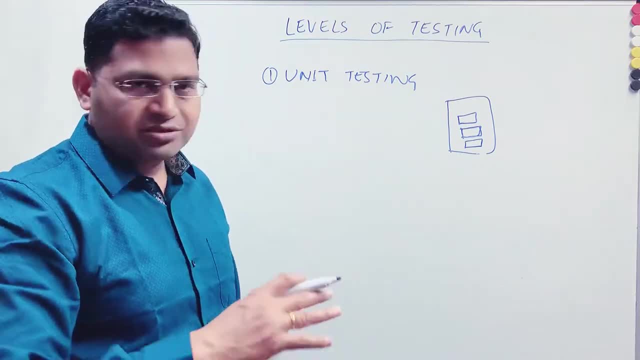 character and those sort of rules might be there right, just just for the sake of example. i'm taking these. so when he works on this username and password field, there will be some, you know, restrictions or limitations, basically in terms of username and password. so if he works on the code and 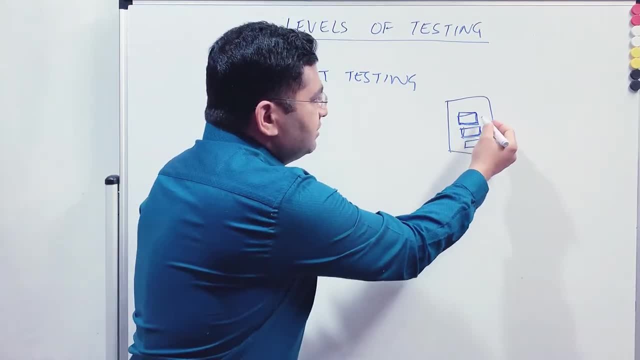 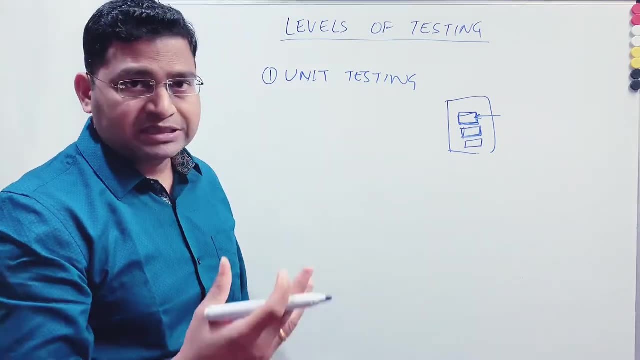 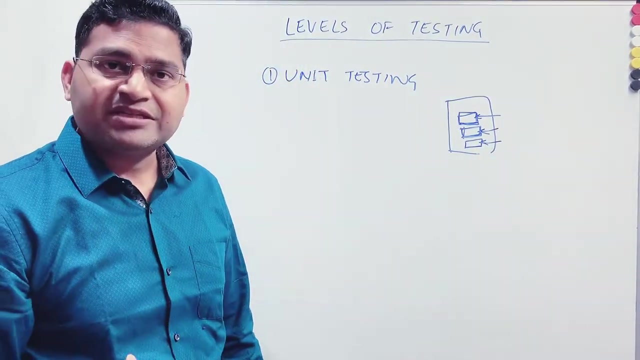 he creates these username and password field. you can think of these as a small units, right, or the you know component. so unit testing is also known as component testing. so these can be you know components or the units that can be tested separately because there is a underlying code. 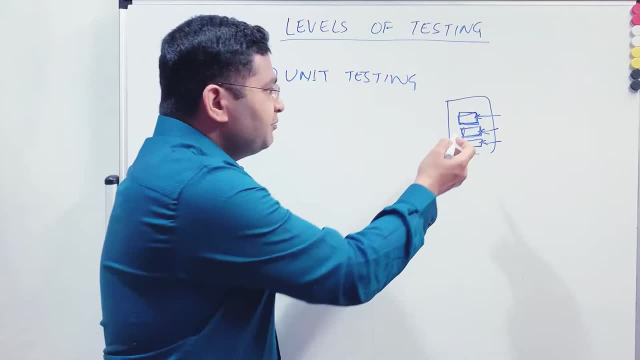 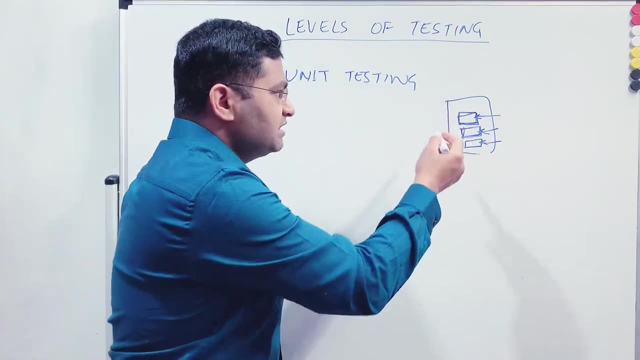 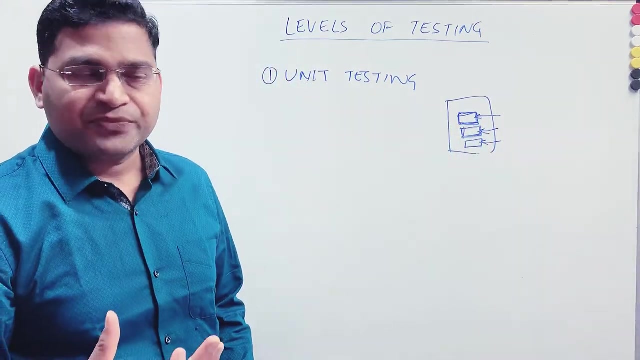 that the developer develops in order to make them visible on the screen as well, as if there is any logic that needs to be built for these units, he needs to build that as well. now, once these in standalone units are built, okay, say, for example, username, he wrote the code and he. 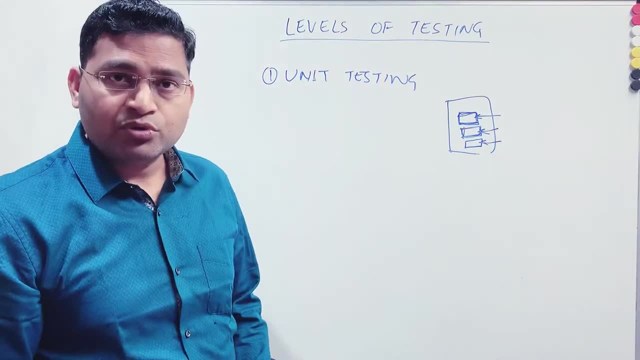 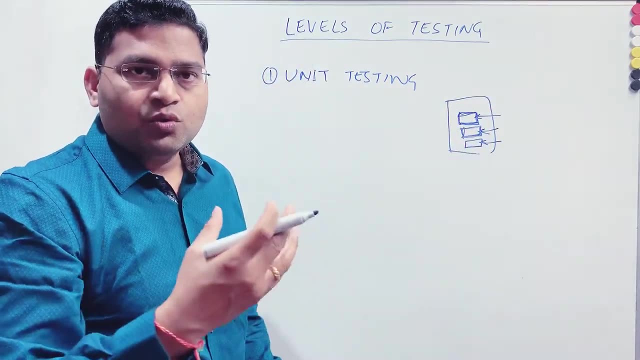 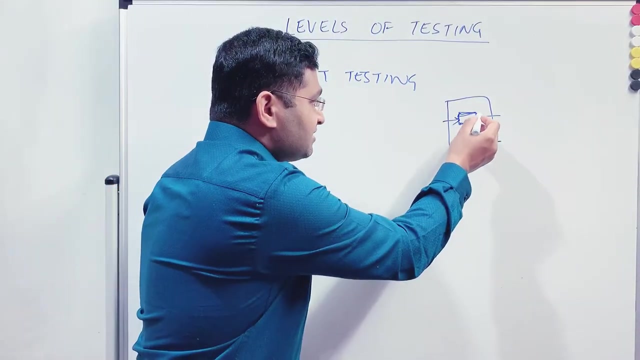 also implemented the logic. that's a standalone unit or component that he has built and then he will be adding that to the overall page, right. so when a developer is testing this particular unit or unit or component, he adds up what he has introduced into that particular function. he says: 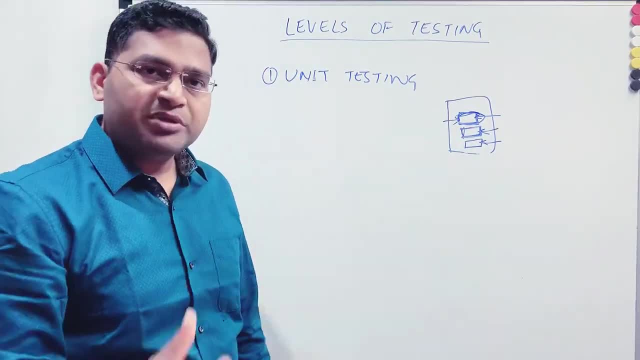 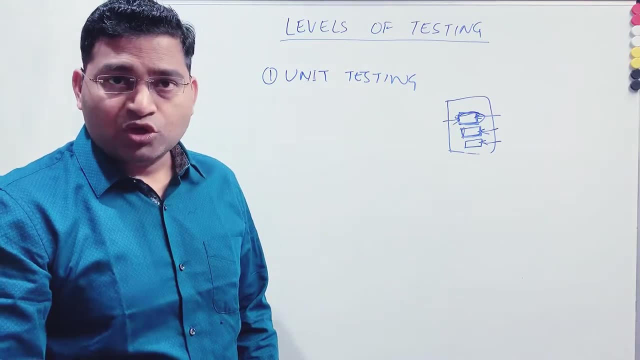 okay. so this farming valor that has been developed today is correct, and if i add this component here, it isEvery tastes a different property, and so that is known as unit testing or unit as a standalone, just say. for example, is testing the only username field with different combinations most of the time. 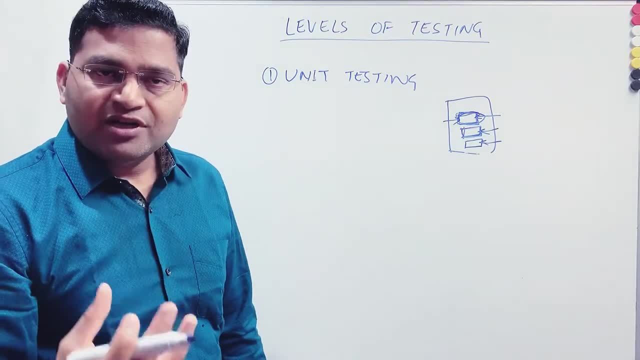 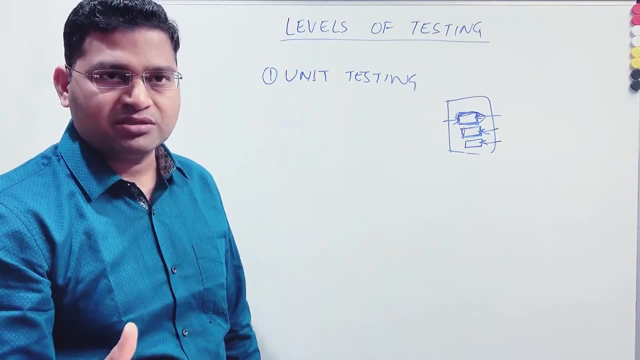 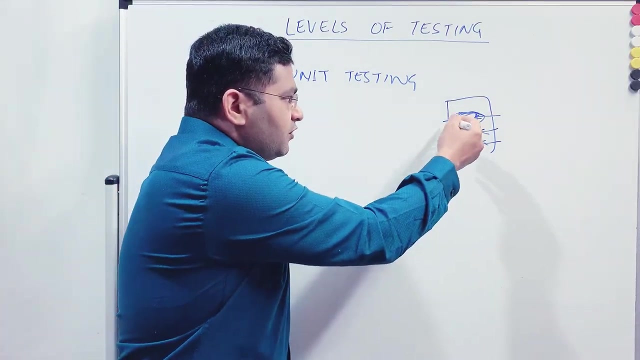 it is, the unit testing will be done by developers themselves. but if you are white box tester, name field will be tested through unit testing tool. For example, you know JUnit is widely used in Java development, with all different combinations and whatever logic has been built for that. 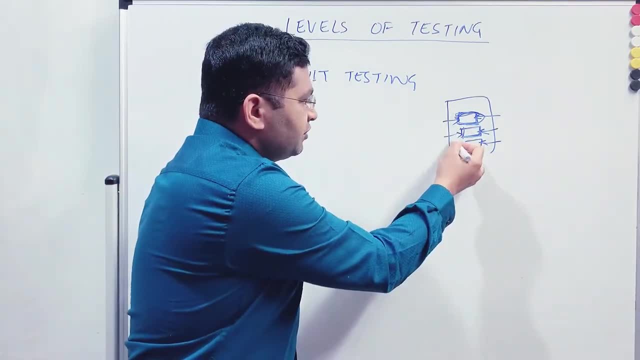 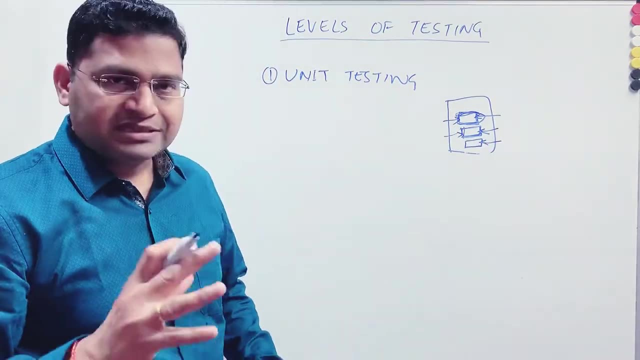 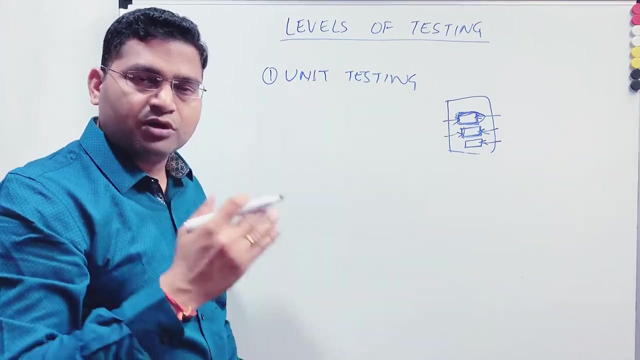 particular unit or the username field. Similarly will be done for the password right. Any other field that is there on the page- that will be tested accordingly. So that's what unit testing is all about. okay, So that's the first level of testing When developer develops those units, or 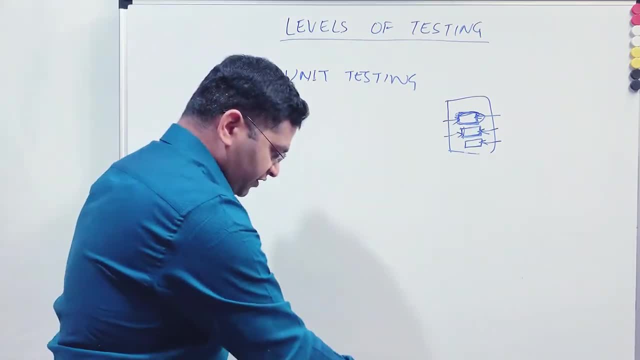 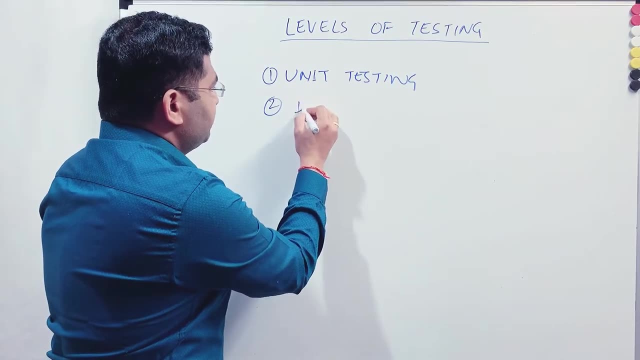 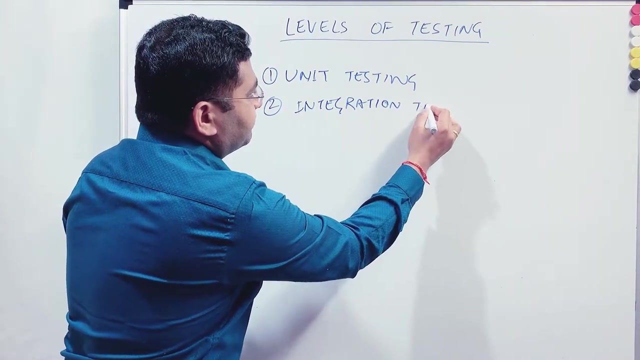 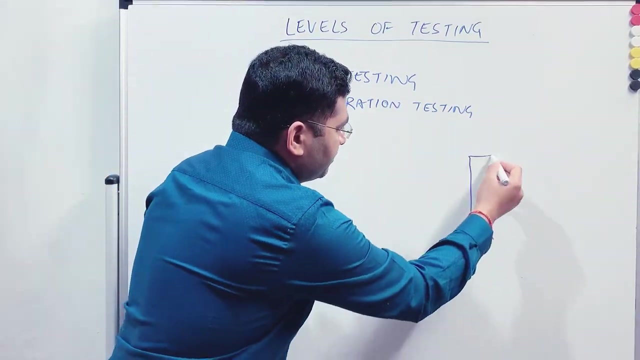 components. he tests or she tests those first, all right, And the next phase is integration. okay, So integration testing. Now what happens in integration testing? So units are built, okay, So on On the page you have the units built. So username field is there, password field is there and the 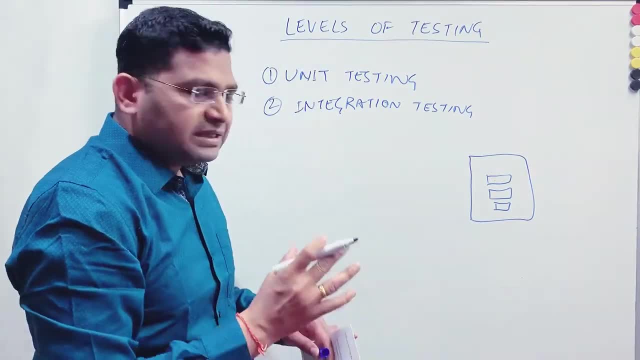 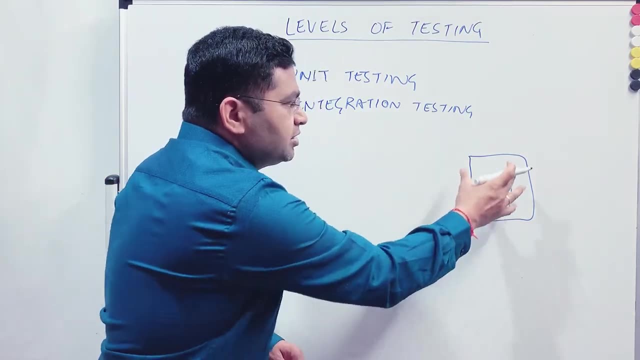 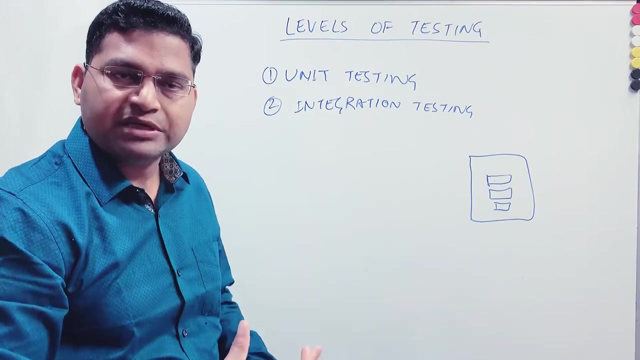 login button is there. okay, So once all these smaller units have been tested and integrated, so basically they are integrated together into one module or one, you know, piece. So this page will be visible, which will have username and password and login button. okay, So this becomes. 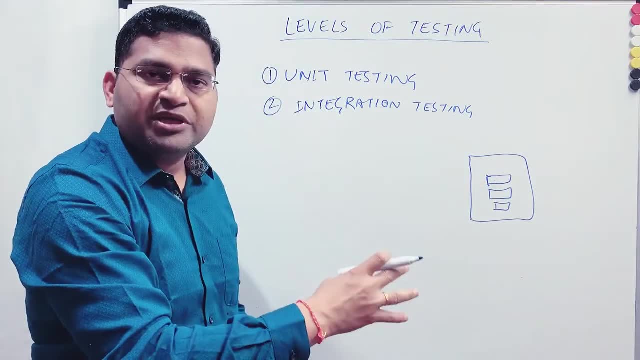 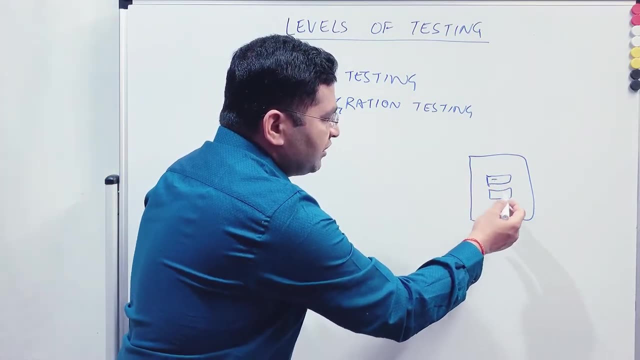 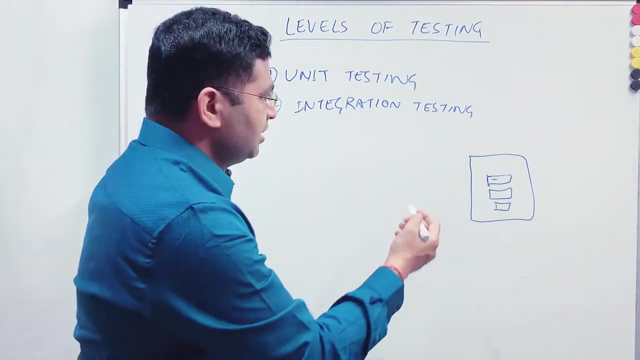 your integrated page, Or integrated page with all the units that need to be there on the page with any business logic, say for example, valid username, valid password, and I click on login, it should show me the login successful message and login should happen successfully, right? So in the integration? 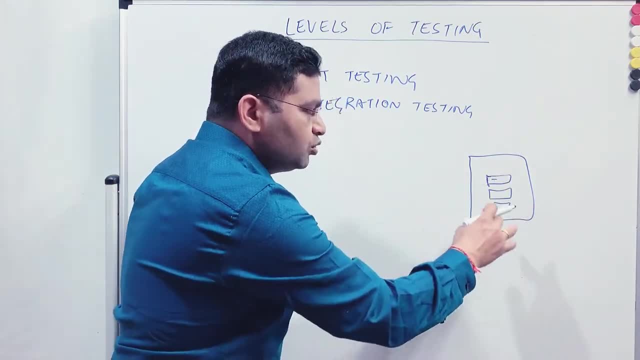 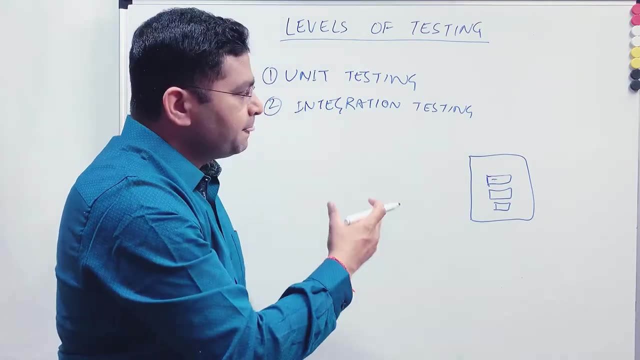 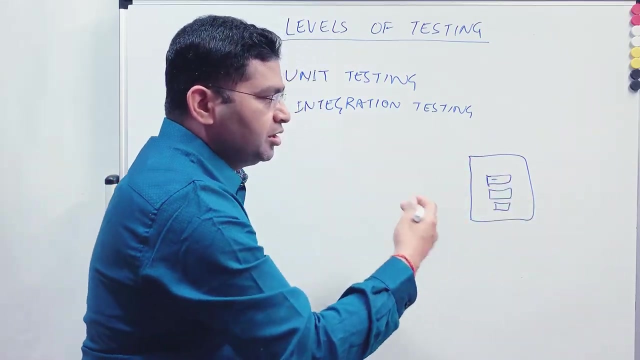 what developer does is they integrate the units that they have developed into one code or logical code that will display this particular page in our example, and integration testing will be done by the person who will be launching this particular page, and then he'll try to test through various 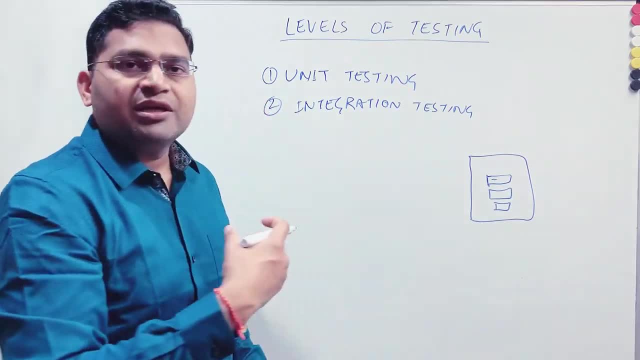 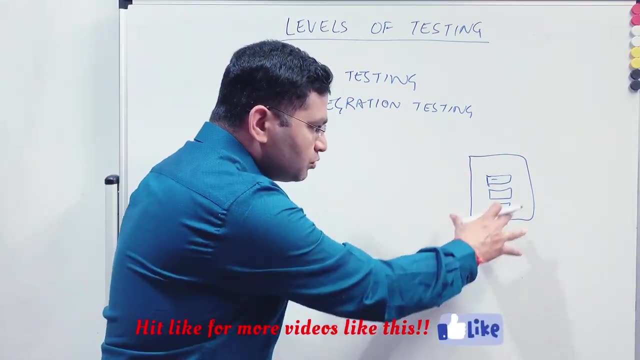 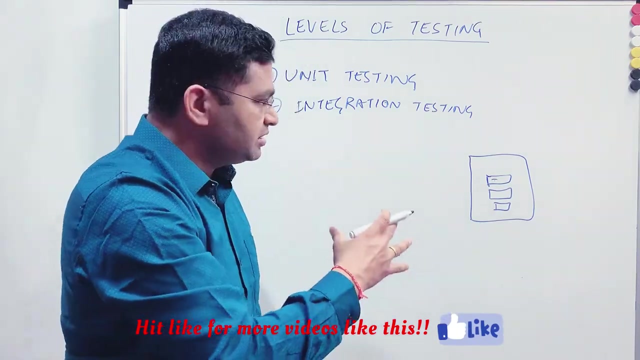 combination of username and password. So valid username, valid password. he'll try to log in Valid username, invalid password. so all those combinations and the business rules that have been implemented on this integrated whole piece or page that will be tested right. So this is. 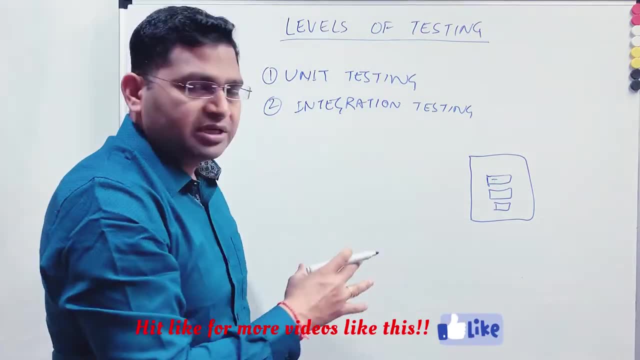 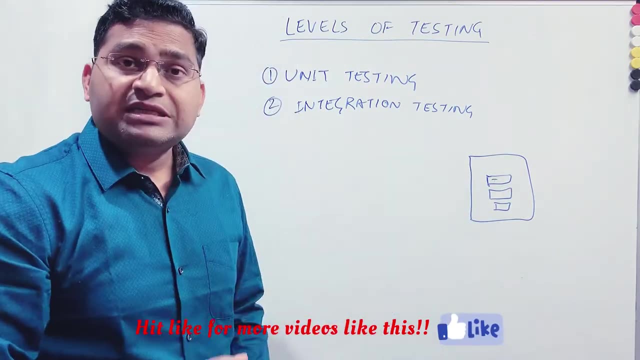 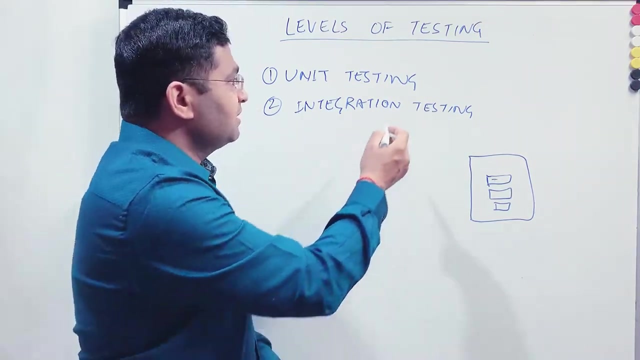 what integration testing is all about and how integrate integration testing in хence. starting. this video will be done for the login page. okay, so this integration testing will be mostly done by the testing team. most of the time, I mean, this is the testing team's responsibility or the testers responsibility. unit testing could be. 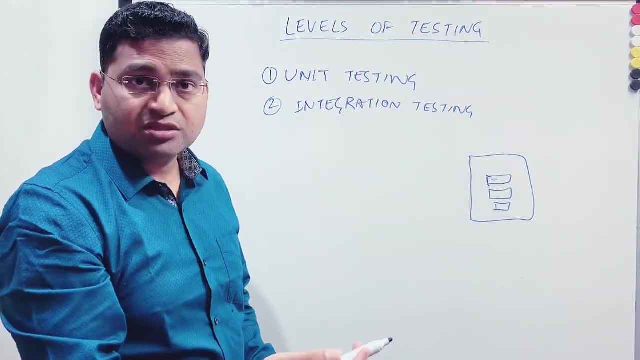 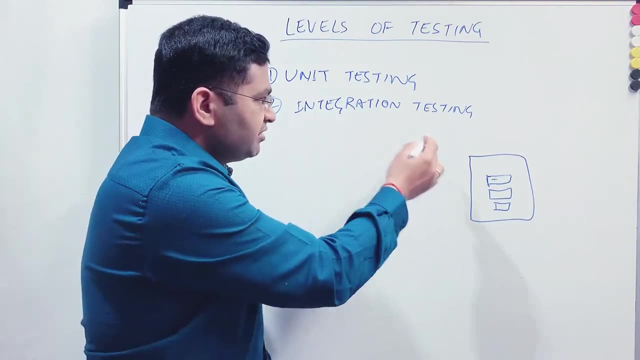 developer could be tester. okay, so it depends: if you're a white box tester, you will do it. if you're, you know, not a white box tester, then development team will do it. but integration testing is the testing team's responsibility and if you're working in the testing team or a tester, you will do the integration. 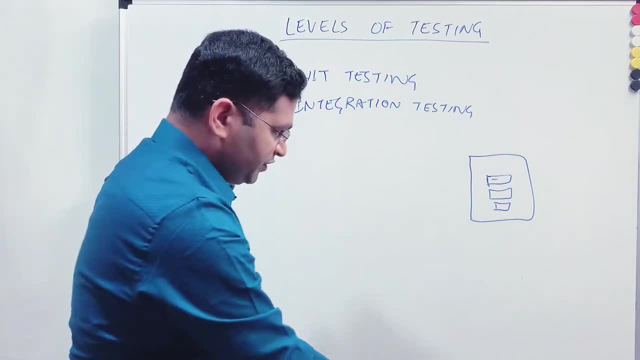 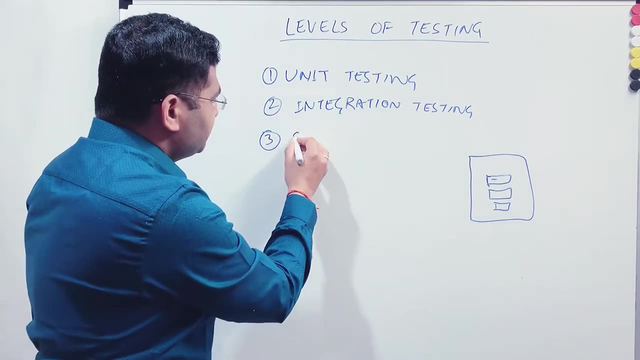 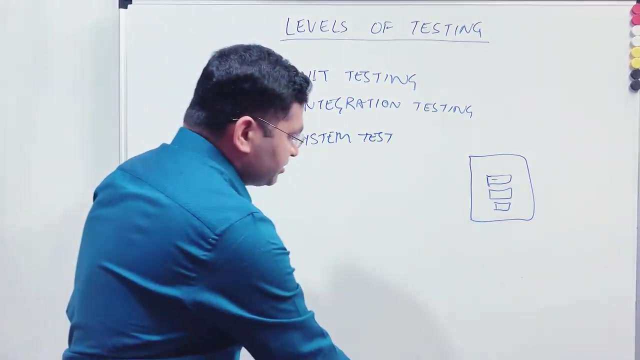 testing of the modules that are being deployed, right? so that's what integration testing is, and that's the next level of testing. the third level of testing is system testing. okay, it's a system test. now, in the system test, what happens is system test. you can categorize into two, mostly, right? so? 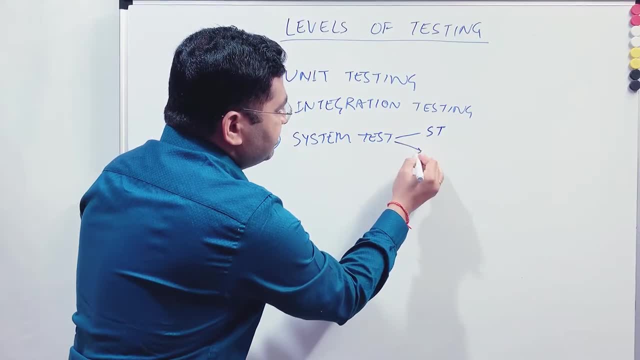 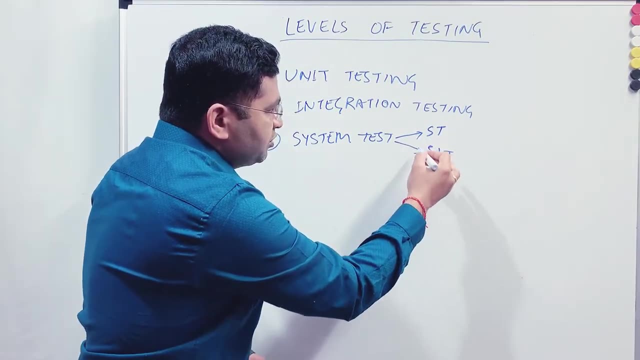 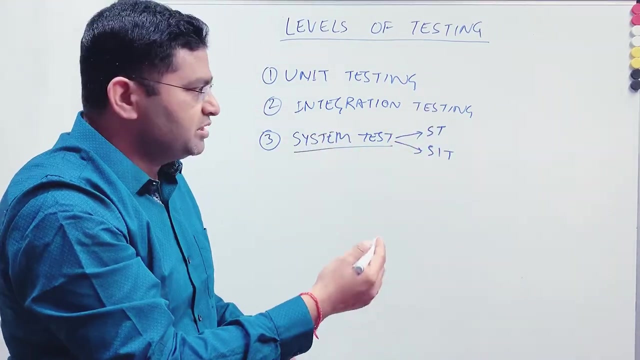 system test, you can say ST, and then there is one which is SIT, which is very, you know, popular. so you need to understand what is the difference between system test and system integrated test. but within system test, these are the two phases that can be possible, depending on how. complex. your software is. so in the system test, what happens is so in the integration testing. say, for example, you just verified the integrated login page which has username and password and login button, right. so that's one integrated model that you verified now in the system test, the overall software. 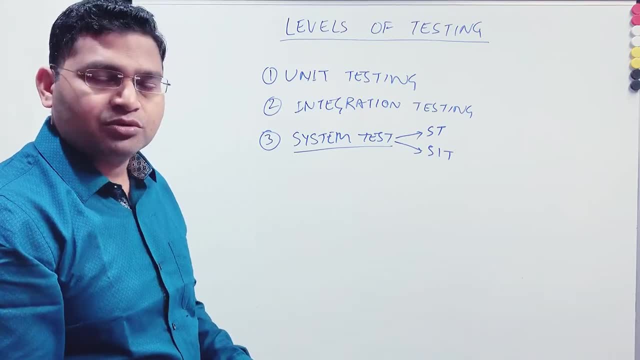 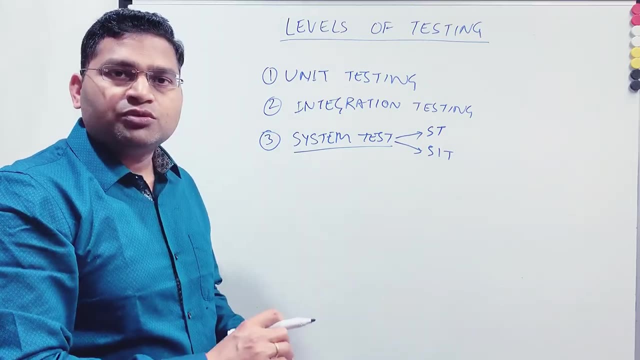 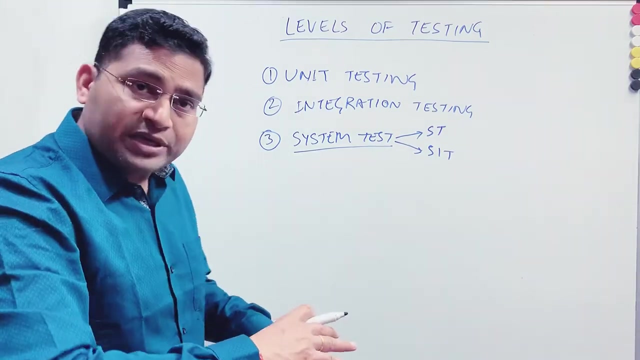 or the overall e-commerce website when it is developed. so you have the login page. once you log in, you add the items to cart, you remove the item from the cart, you go to the checkout page, you make the payment and all things work successfully right? so that's when all the modules are built and integrated as 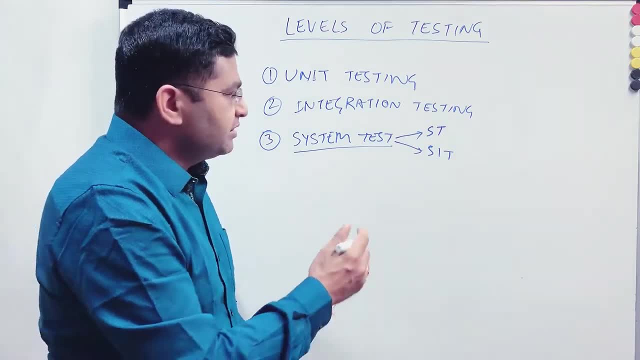 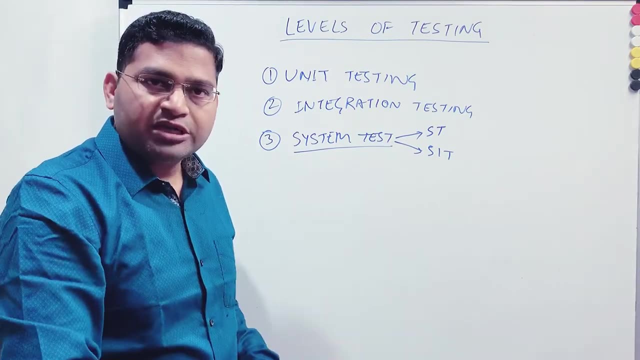 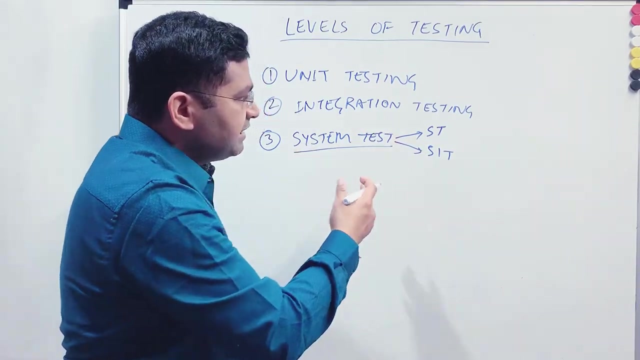 a system or a system as a whole, then that's what system testing is all about. okay, so once everything in the software is ready and deployed, then that's when system testing starts, and this is also done by the testing team. now system testing can have a system. 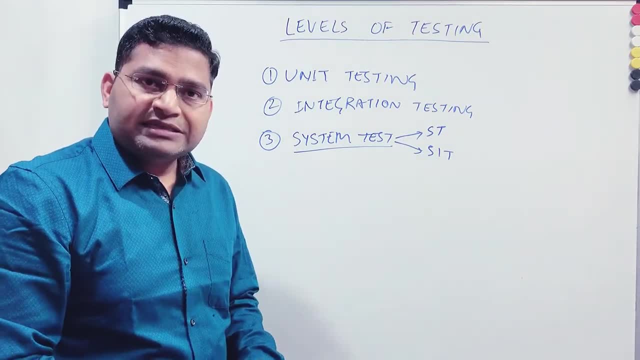 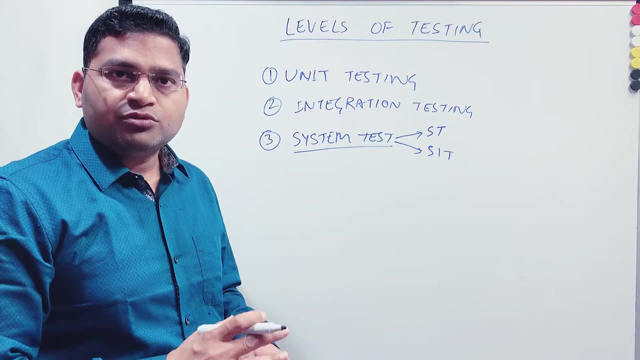 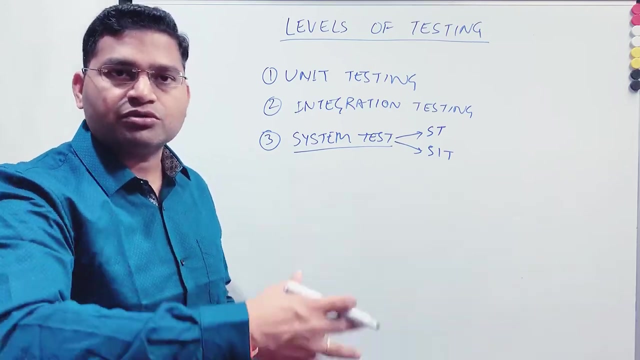 test phase. if your software is a standalone software or it doesn't integrate with any of the external systems, right. so say, for example, you have a software that runs on a standalone machine and doesn't integrate with any other. you know machine or softwares. okay, so that. 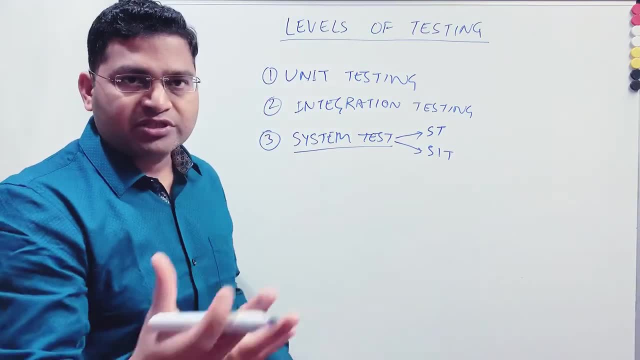 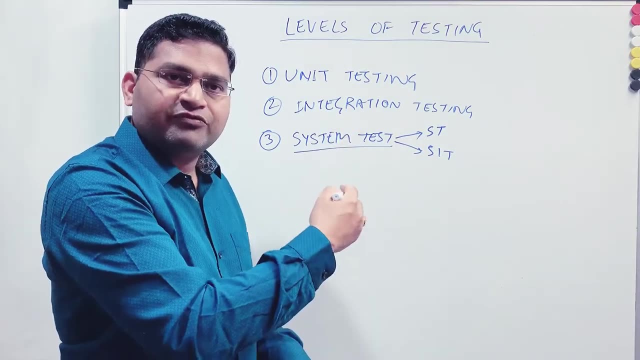 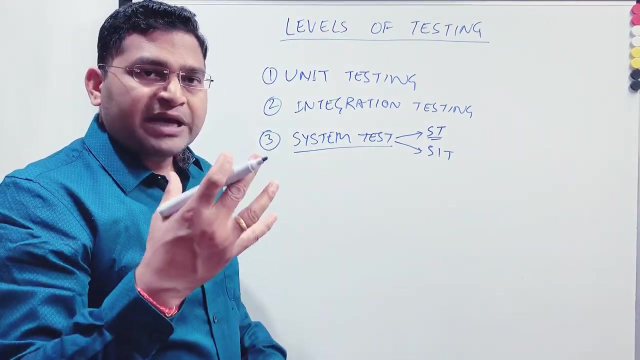 is what will be done as a system test. for example, you have the Microsoft Word document is a standalone software when it tests that, that system testing phase will just have that ST system test phase. but say, for example, you are working in the banking application, so banking application might have 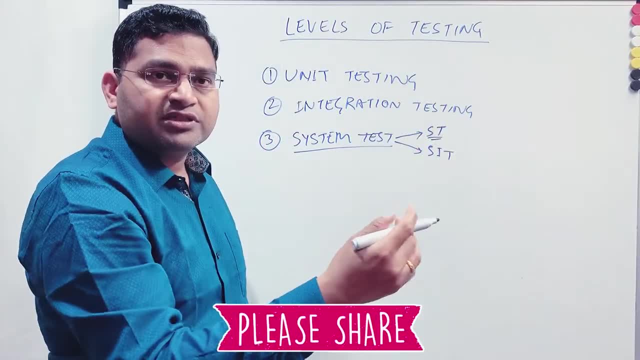 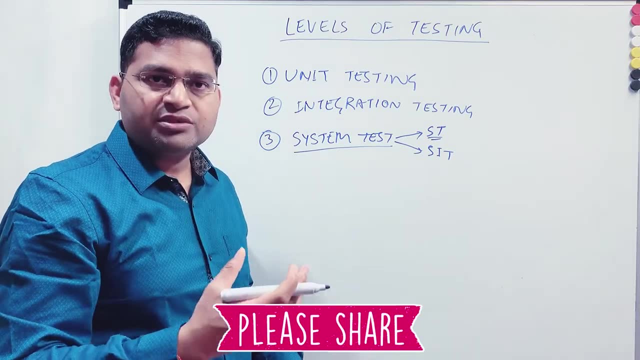 integration with external systems as well, say, for example, when I apply for the car. for example, when I apply for the car, for example, when I apply for the car, Then after application of the card, when card is received or card is being embossed and sent to me, that is done by the third party, you know. vendor. 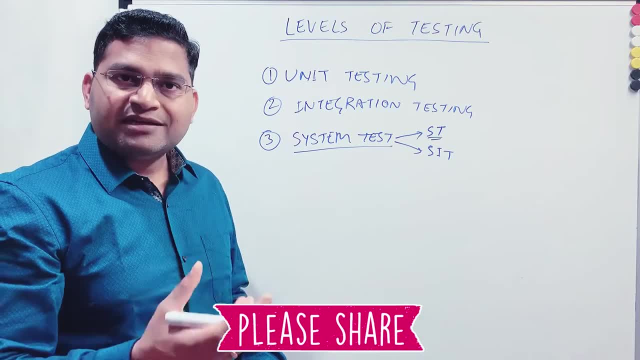 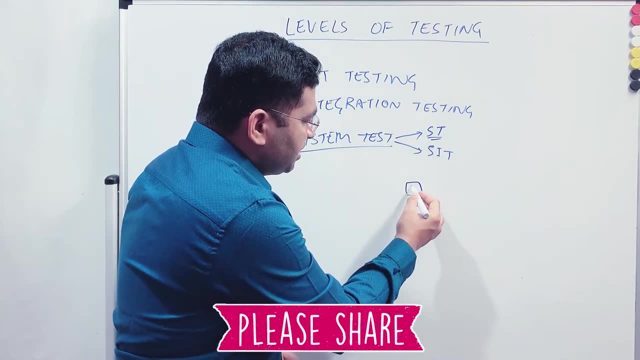 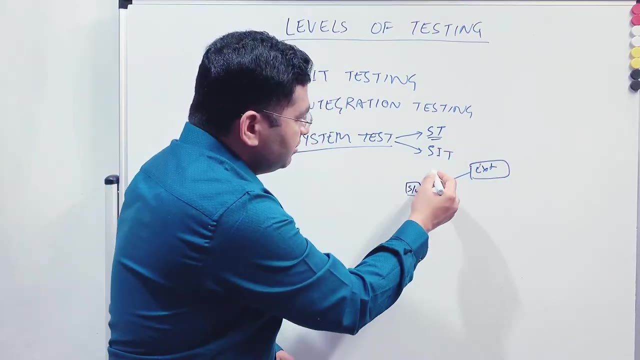 It might be possibilities done by third party vendor who send me the physical card or the chip right. So when that's the case, when my software say, for example, my software here, is integrating with some of the external systems as well, then I have to do SIT as well, system integration testing okay. 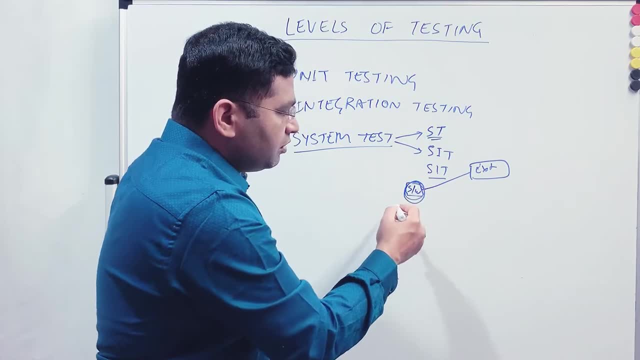 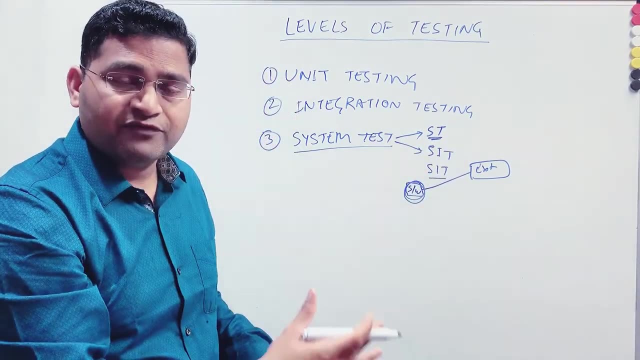 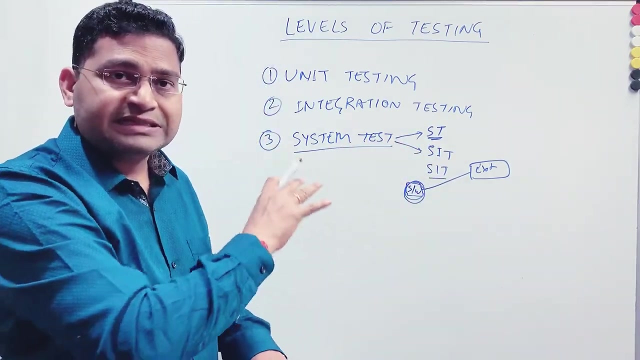 So in that case this is not a standalone software that runs on my machine. So that is why in system test phase there will be ST and SIT, both, If your software or application integrates with external Systems. I'll explain these two in a lot more detail with real example in upcoming tutorials. 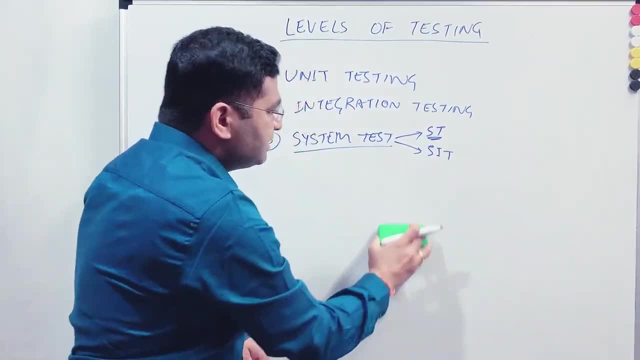 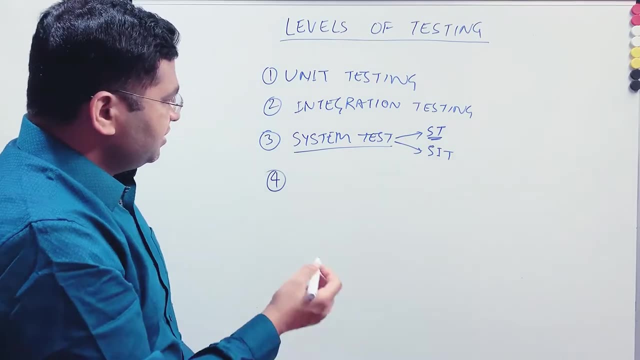 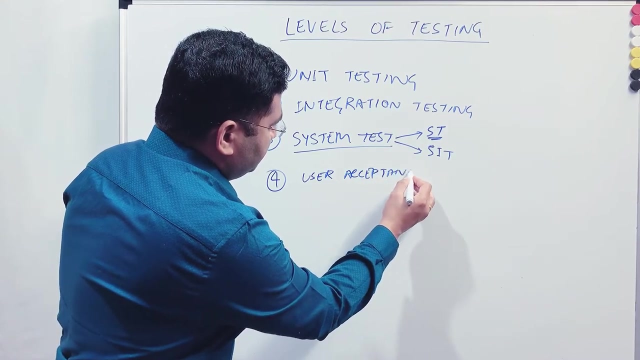 So don't worry about those in detail at the moment. So this is the next level of testing. So system testing is the next level of testing. Now the fourth level of testing is user acceptance testing. All right, Now, what happens in user acceptance testing? 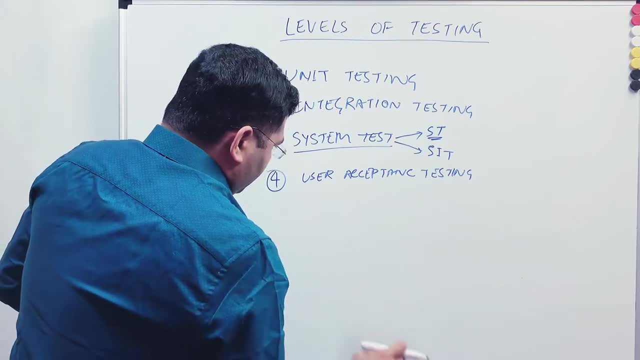 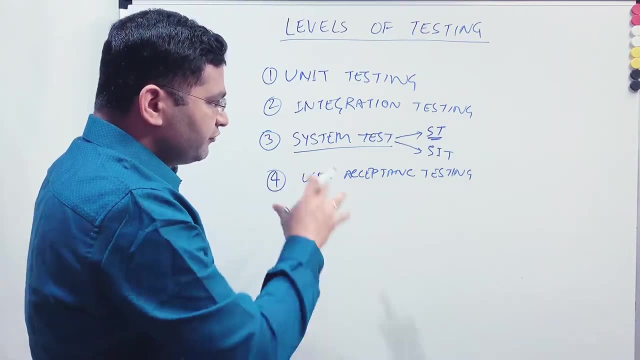 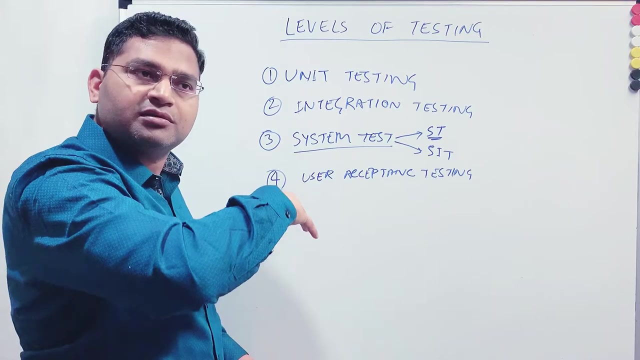 The third level of acceptance testing is the acceptance testing. I'll say so. in the acceptance testing, what usually happens is when the software is being built. the acceptance testing is mostly done by the business- Okay, by the business or by the customer, the real consumer who will be using the software? 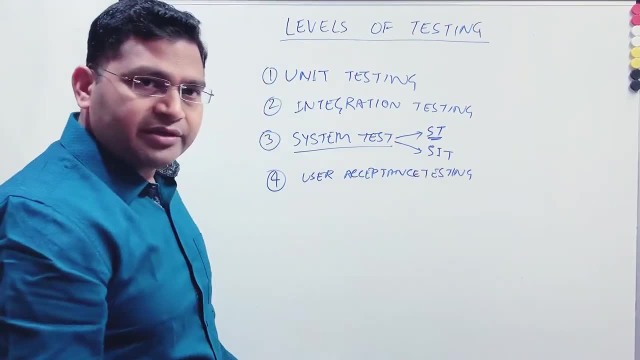 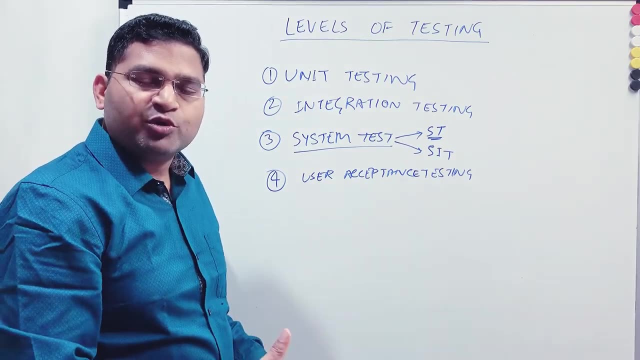 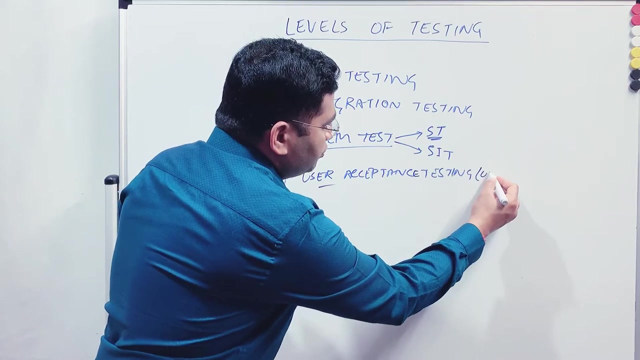 So in the acceptance testing it is mostly seen whether the software that has been built is fit for use or whether it works, provides the real value or it provides the functionality that the customer is looking for. and that is why this is called as UAT- user acceptance testing- in short, it is called UAT. 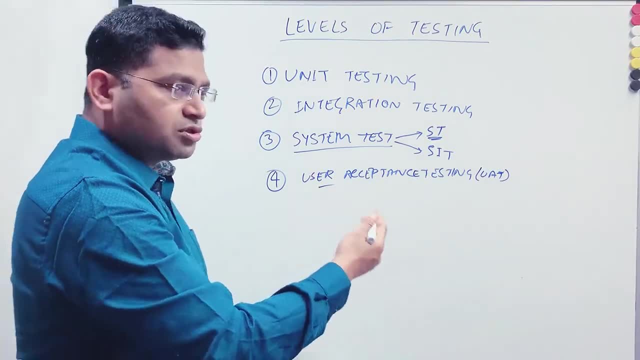 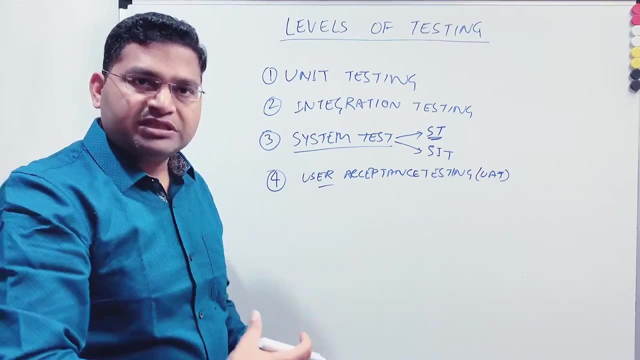 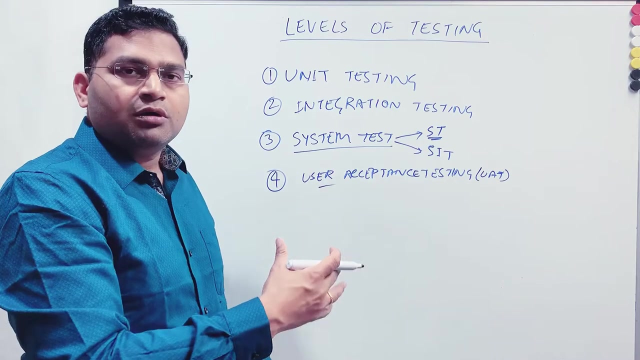 and user acceptance testing, because user, who is the user of the software, will be testing it and whether he'll, you know, accept it or reject it, or he'll raise the defect that this is not what I was looking for. and then the team needs to fix those or make sure that the software that has 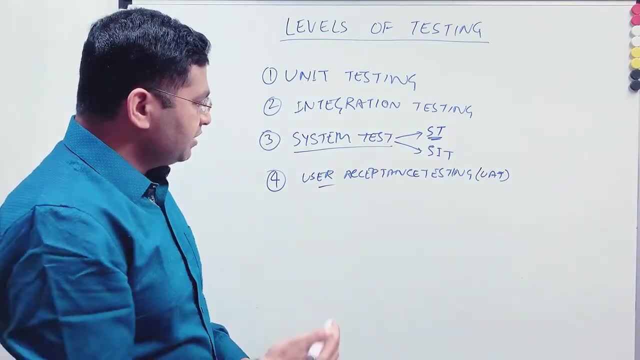 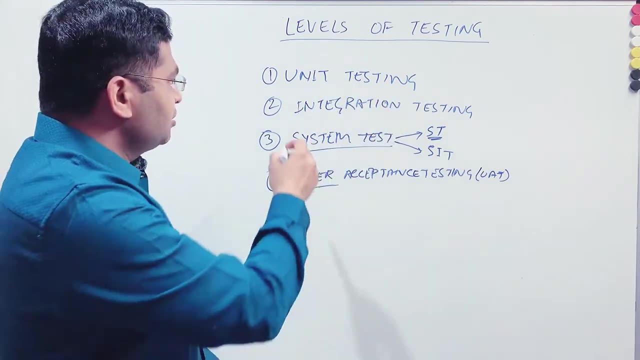 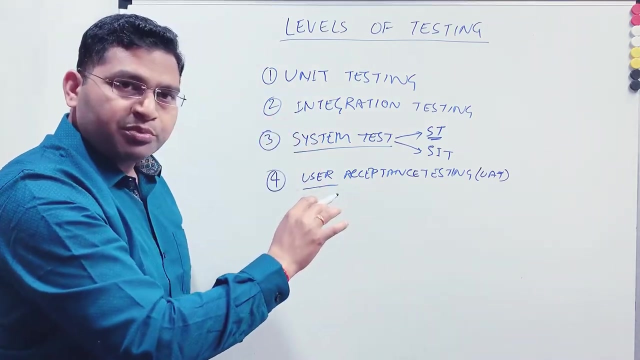 been developed meets the actual user requirement, right. so this is the next phase of, or the level of testing, right? so these are the four levels of testing that you need to remember for any interview purpose or for getting into, you know, even if you're working in the software testing field. 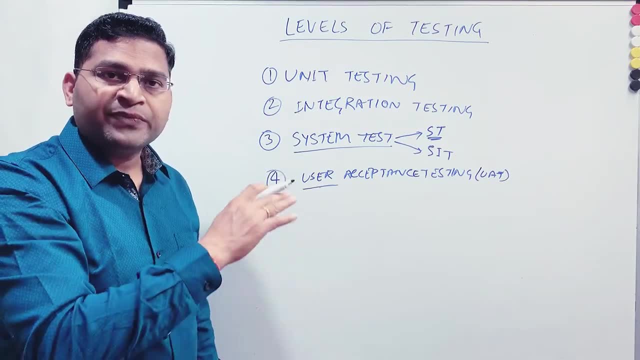 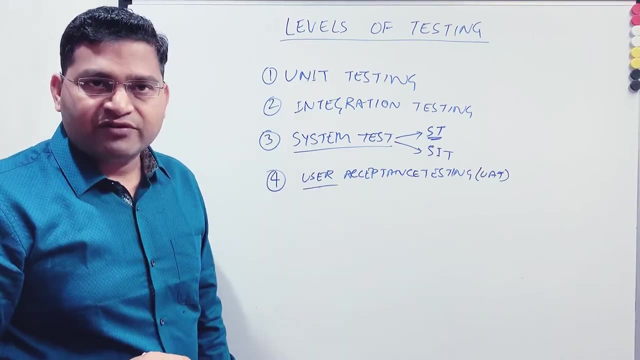 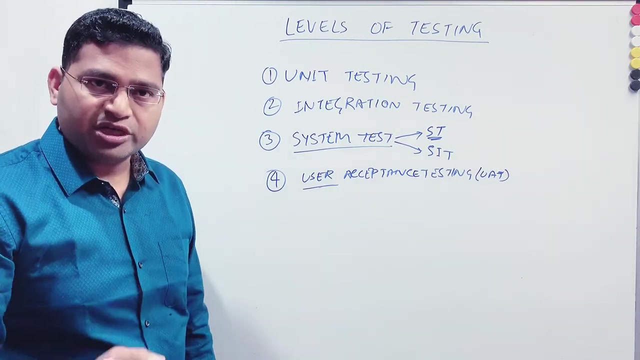 you need to. you need to understand these levels, because when you understand these levels, you will be able to understand how you are going to segregate your testing effort, based on the development cycle, and when the, the delivery or the code is being deployed into the, into the test environment. 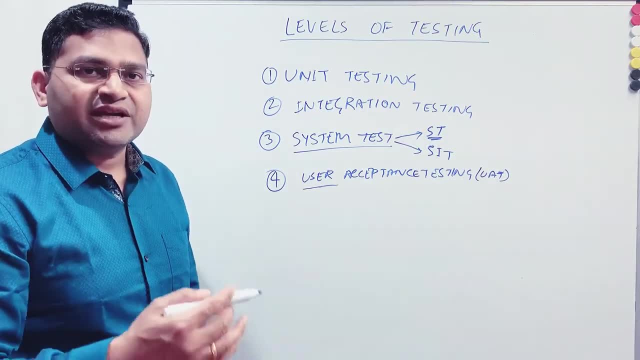 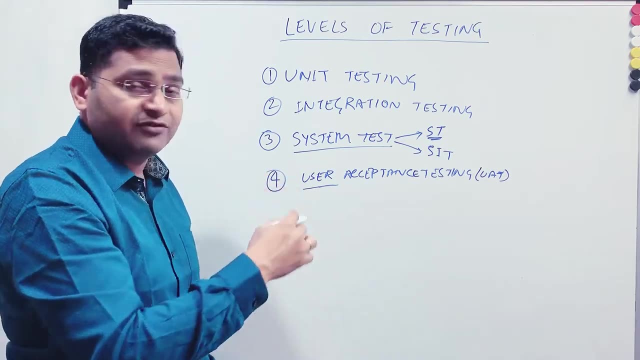 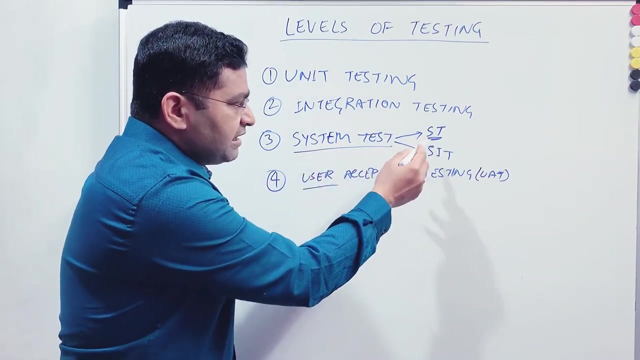 you will be able to write the relevant test cases and test accordingly when you have the knowledge of levels of testing and what level what you need to do in each level of testing, right? so this is about the level of testing. very important aspect is the system test. it can have just system testing or it can have a